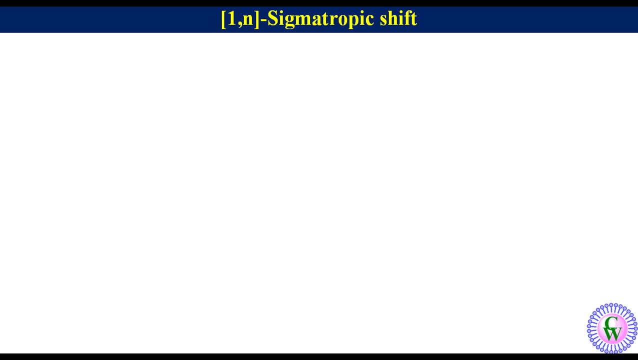 Hello friends, today we are going to discuss sigmatropic shift or sigmatropic reaction. It is a very important topic. There are several types of sigmatropic shift, but in this lecture we will focus only on 1N sigmatropic shift. We will discuss the following points: general: 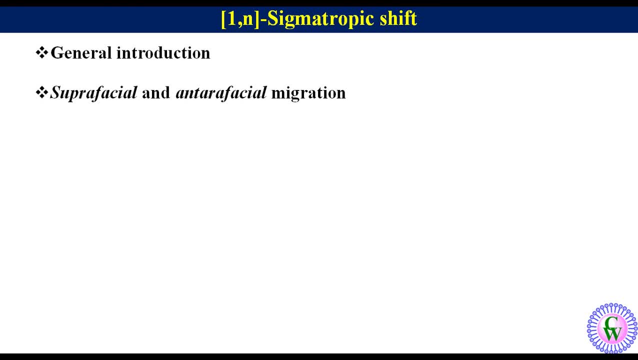 introduction: supra and antirefacial migration rules governing 1-3 H-shift and 1-3 C-shift. rules governing 1-5 H-shift and 1-5 C-shift. and rules governing 1-7 H-shift and 1-7 C-shift. 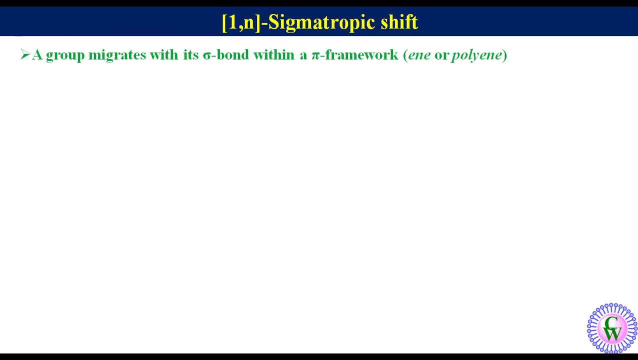 In a sigmatropic shift. a group migrates with its sigma bond within a pi framework like ene or polyene. The migration is accompanied by a shift in pi bonds. Suppose we have a system like this where m is equal to 1,, 2,, 3,, 4, etc. During. 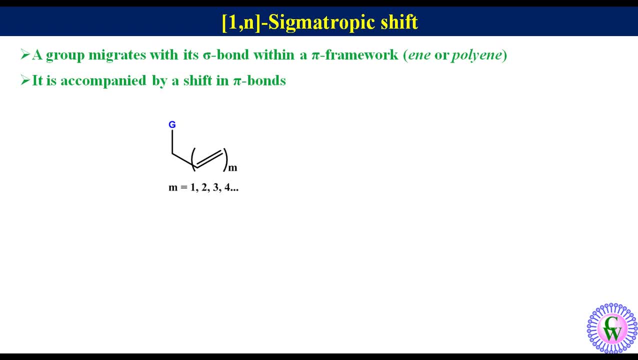 a sigmatropic shift, group G with its sigma bond will migrate to this carbon and this migration will be accompanied by shifting of pi bond. In this lecture we will focus only on 1N sigmatropic shift. The numbers in the bracket have special 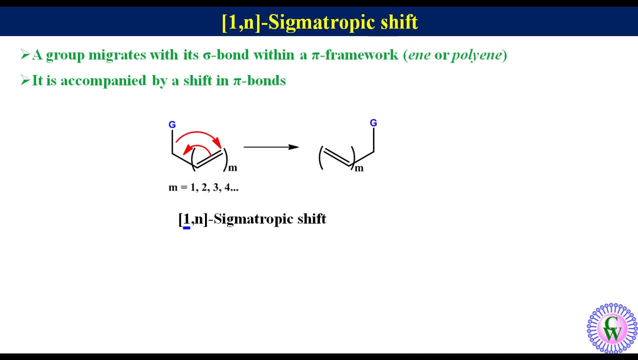 meanings. The left side number, which is 1 in this case, suggests that the group is bonded through the same atom in the reactant and the product. The right side number, which is N, suggests that the number of carbon, which is 1 in this case, is 1 in the reactant and the product. 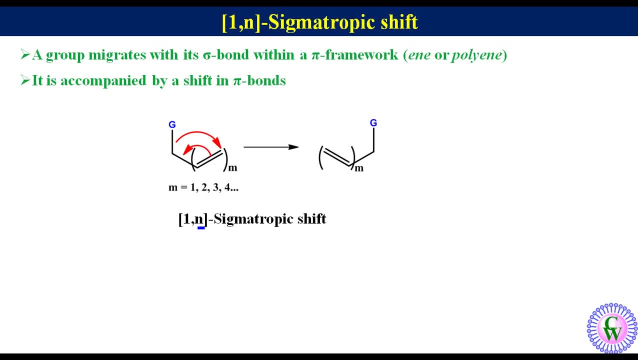 There are 2 Sketches: 1-Items of the pi framework to which group G is migrating. N can be 3,, 5,, 7, etc. G can be hydrogen, carbon or other items, Based on whether the migrating atom is hydrogen. 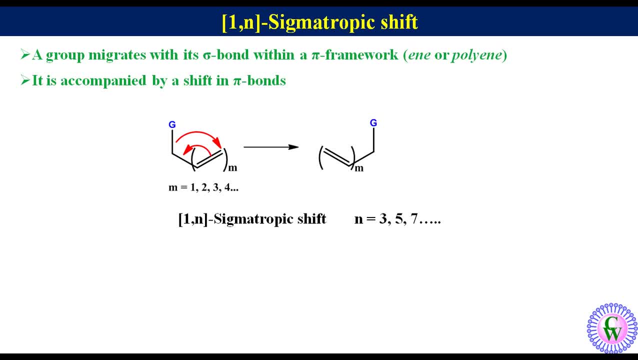 or carbon, and N is 3,, 5 or 7.. 1n-sigmatropic shift can be classified as 1,3-h shift, 1,3-c shift, 1,5-h shift- 1,5-c. 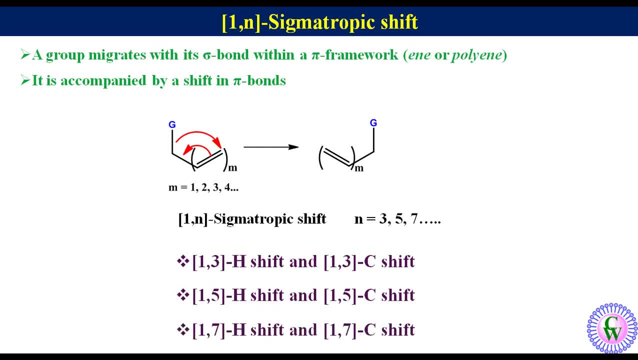 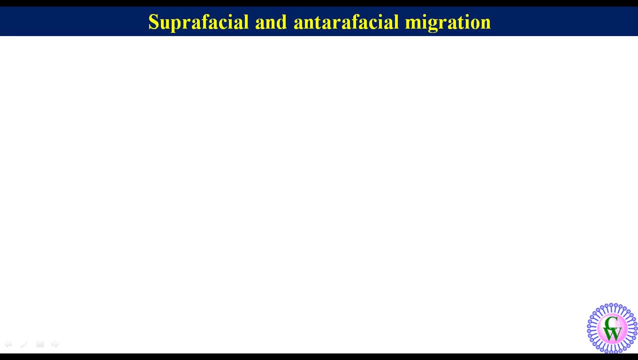 shift, 1,7-h shift, 1,7-c shift, etc. Now we will discuss two terms: suprafacial and enterofacial migration. Suppose we have a system that can undergo sigmatropic shift. The symmetry of the terminal orbitals is like this, and here is the migrating group. 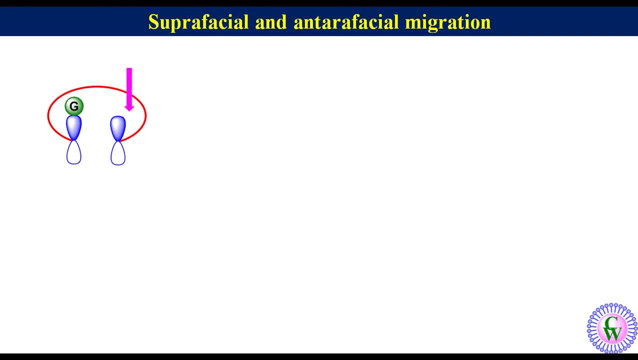 There are two faces of the pi system: top face and bottom face. Here the group is on the top face. If we allow it to migrate, it will migrate to the right lobe, keeping it on the top face. This type of migration, in which a group migrates on the same face of the pi bond, is called 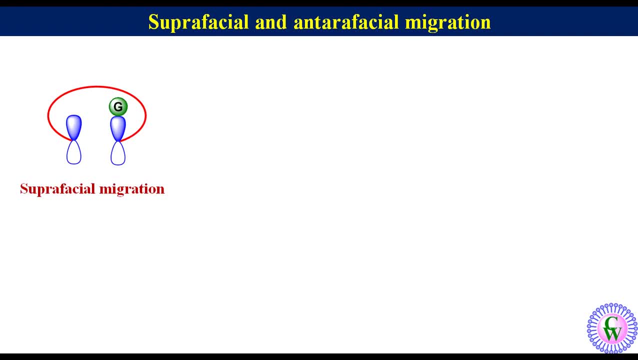 suprafacial migration. Lets have a different case in which the symmetry of the terminal orbitals is like this: The migrating group is on the top face. If we allow it to migrate, it will migrate to the right lobe on the bottom face, like 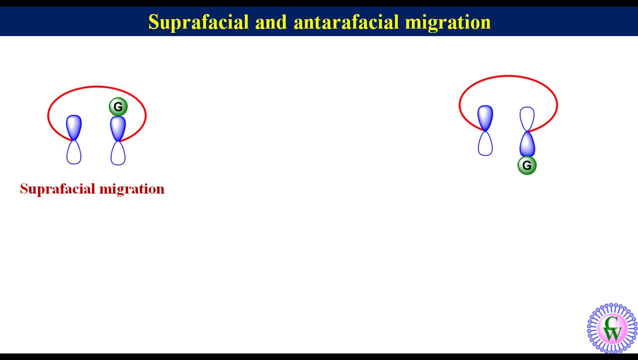 this. This type of migration in which a group changes the face during the migration from one terminus to other, is called enterofacial migration. Lets first discuss 1,3-h shift. According to the definition in 1,3-h shift, a proton should migrate to the third carbon. 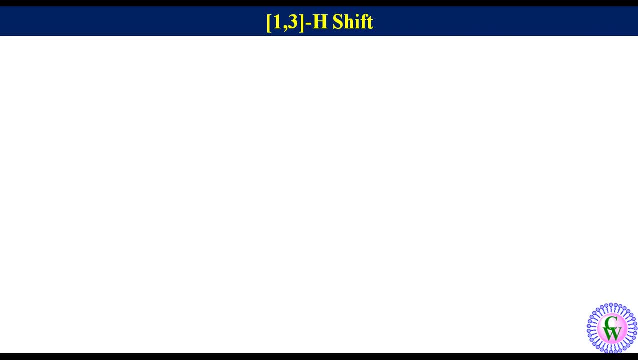 from the carbon of its attachment in an allylic system. For the discussion about under which condition which type of migration is allowed, lets take the example of simplest system, which is propene. Even though it is a pericyclic reaction, it is assumed that it is proceeding through allylic 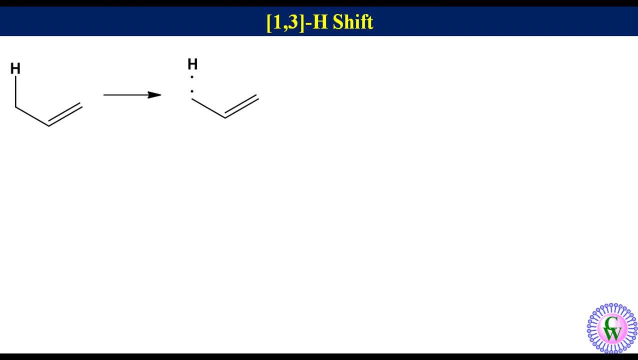 radical for the purpose of easier explanation. Under thermal condition, the HOMO of allylic radical has C2 symmetry like this: The HOMO of allylic radical has C2 symmetry like this: The HOMO of allylic radical has C2 symmetry like this: 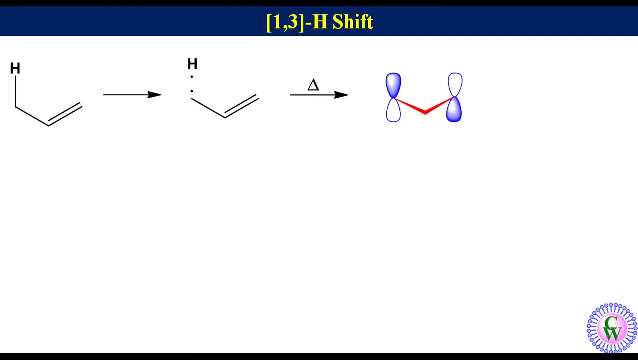 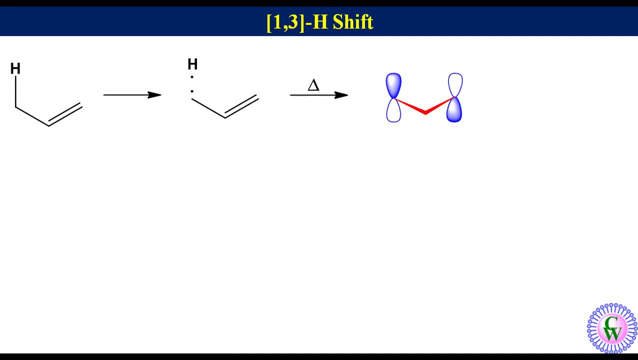 Here. I am not going to discuss how to draw the structure of HOMO, as I have uploaded a separate lecture on this topic. The link for the same is given in the description Here. this is the hydrogen. We can clearly see that it will opt enterofacial migration through this transition state. 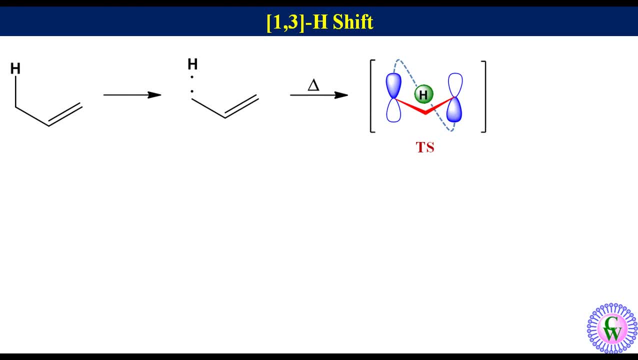 This transition state is so straight, So strained to be formed, So strained to be formed And therefore one-three-edge shift is thermally not allowed Under photochemical condition. the HOMO will have 패symetry, like this Means it will have sigma plane and will not have C2 symmetry. 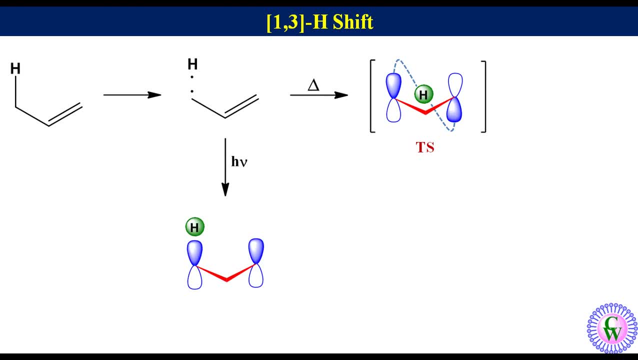 Here is the hydrogen atom. We can see that it will opt suprafacial migration through this train. We can see that it will opt suprafacial migration through this train. We can see that it will opt suprafacial migration through this train. 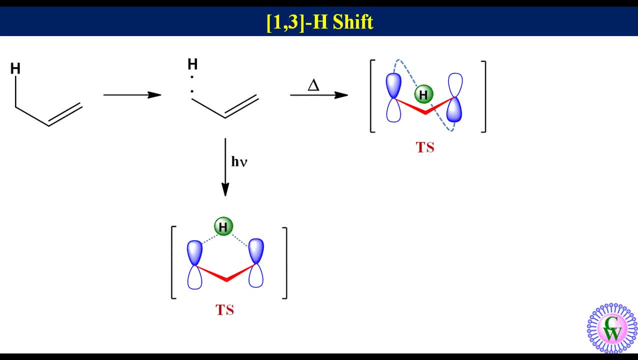 That's why it is between TiO and occupied united тан viaje transition state. Because of a smaller size of the hydrogen atom, it cannot bind simultaneously to overlap with the two p orbitals. So we can summarize: under thermal condition 1,3-H-SHIFT is anterofacial and not feasible, while under 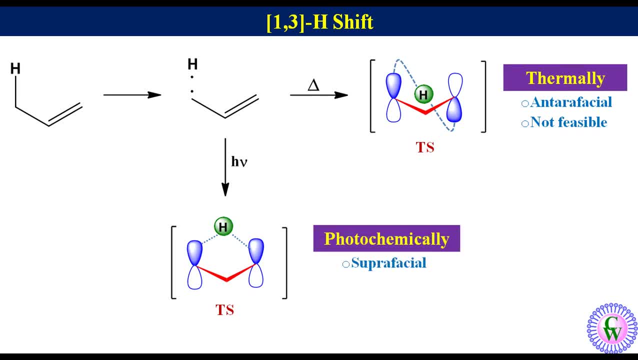 photochemical condition. it is supra facial and also not feasible. 1,3- carbon-shift: According to the definition in 1,3-carbon-shift, a group migrates to the third carbon from the carbon of its attachment. For the discussion, under which condition, which type of migration is allowed? let's take 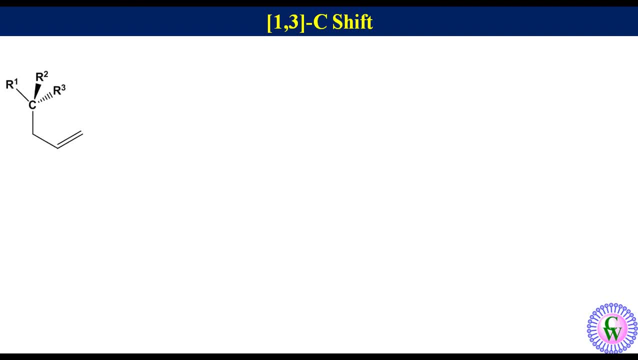 the example of a hypothetical propene derivative. In this case too, we will assume that it is proceeding through allylic radical. Under thermal condition, the homo of allylic radical has C2 symmetry. like this: Here is alkyl group. In this case, despite C2 symmetry of homo of pi. 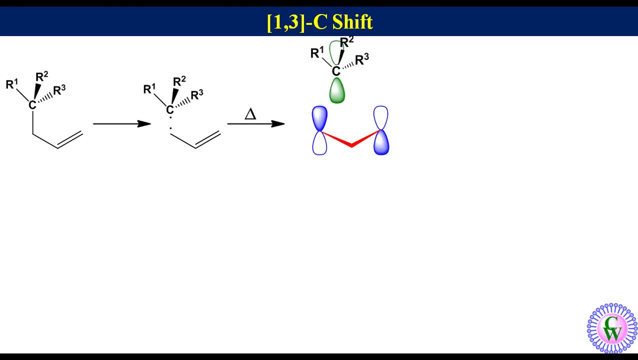 framework alkyl group can migrate supra facially to generate this strong transition state because the p orbital of the carbon, due to the presence of two lobes, can overlap with the orbital lobes of both the termini of pi framework simultaneously. This transition state will collapse into product with the 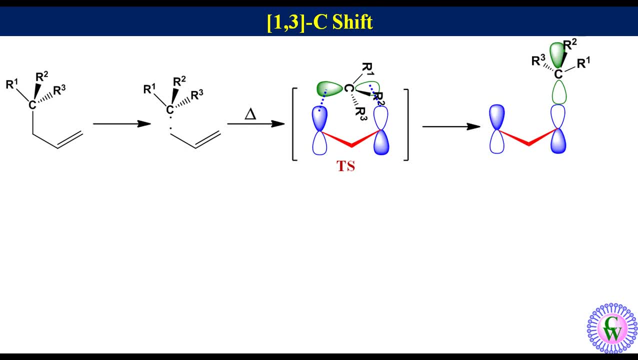 inversion in configuration of the migrating group. Under photochemical condition, the homo of allylic radical will have symmetry like. this means it will have sigma plane and will not have C2.. Here is alkyl group. We can see that in this case too, it can opt supra facial migration to generate this transition state in which 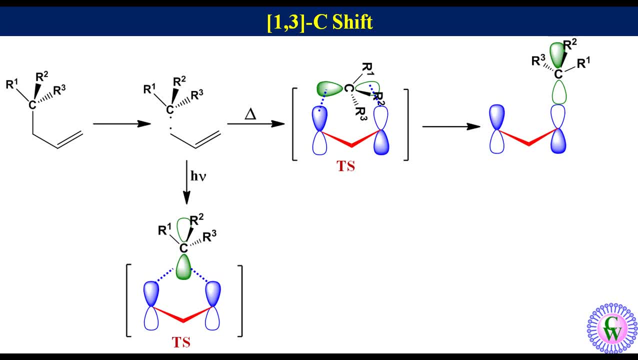 one lobe of the p orbital of the migrating carbon overlaps with the orbital lobes of both the termini of pi framework simultaneously. This transition state will collapse into product that has retention in the configuration of the migrating group. So we can summarize under thermal condition: 1,3-carbon shift. 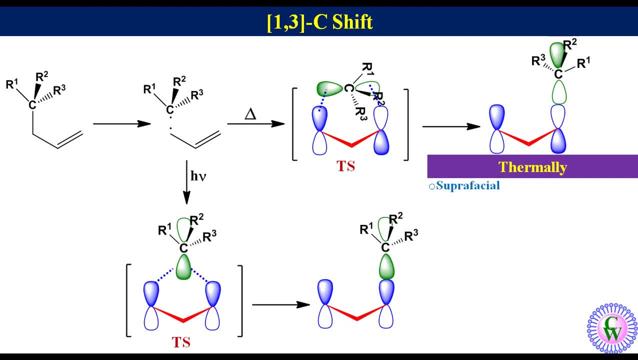 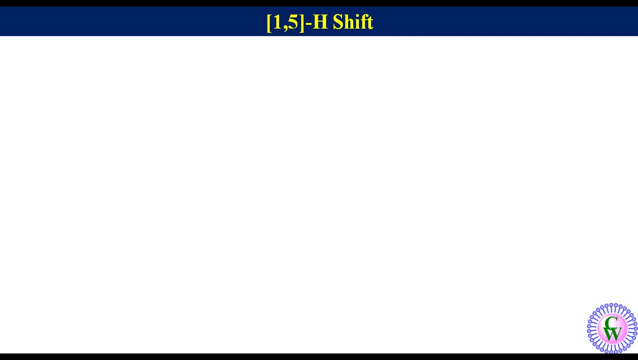 it is suprafacial and feasible with inversion in configuration of the migrating group, While under photochemical condition it is superficial again and it is feasible, but with the retention in the configuration of the migrating group: 1,5-H shift. In 1,5-H shift a proton should migrate to the fifth carbon from the carbon of. 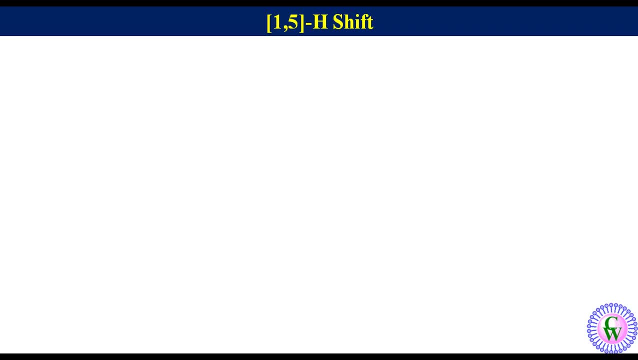 its attachment in a pentadiene system. For the discussion about under which condition which type of migration is allowed, let us take the example of the simplest system, which is 1,3-pentadiene. Let us assume that it is proceeding through 1,3-pentadienyl radical. Under thermal condition. the HOMO of the pentadiene radical has placed a proton in the pentadiene system. So the HOMO of the pentadiene radical has placed a pentadiene of symmetry like this: Here is hydrogen. We can see that it will opt superficial migration. through this transition state. Unlike transition state of 1,3-H shift, this transition state is stable and therefore 1,5-H shift is thermally allowed Under photochemical condition. the HOMO is stable. This transition state is very strained. Therefore 1,5-H shift is photochemically not allowed. 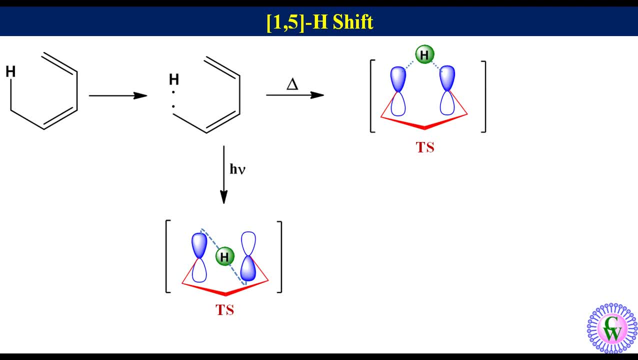 So we can summarize: Under thermal condition, 1,5-H shift is superficial and feasible, while under photochemical condition it is enterofacial and not feasible. 1,5 carbon shift. In 1,5 carbon shift, a carbon migrates to the 5th carbon from the carbon of. 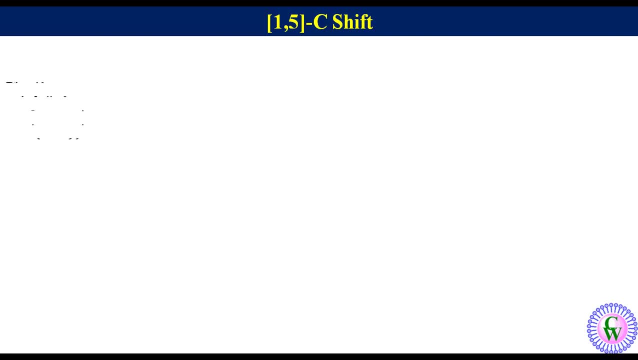 its attachment. Let's take the example of a hypothetical diene. Assume that it is proceeding through the pentadiene radical Under thermal condition, the homo of this pentadiene radical has plane of symmetry like this Here. this is alkyl group. We can see that alkyl group. 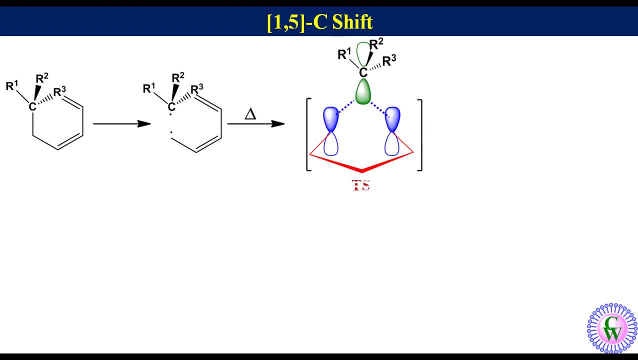 can migrate superficially to generate this transition state in which one lobe of the p-orbital of the carbon overlaps With the orbital lobes of both the termini of pi-1 framework simultaneously. This transition state will collapse into product with the retention in configuration of the migrating 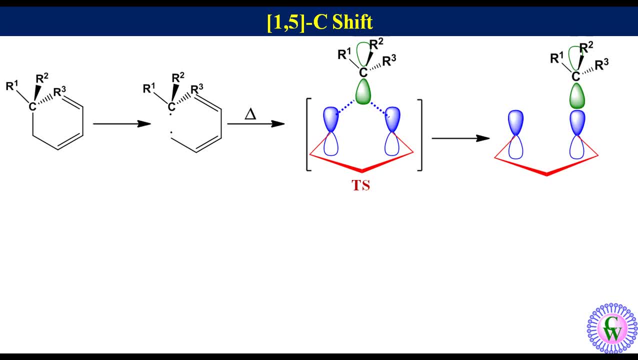 group. Under photochemical condition, the homo of the radical will be cytosymmetric like this: Here is alkyl group. We can see that in this case too, the homo of the radical can opt superficially to generate this transition state. Under thermal condition, this homo 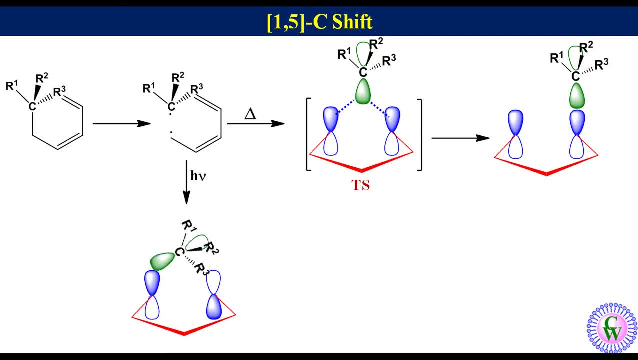 of the captain will migrate to N Expert for Woah, So it can opt superficial migration to generate this transition state in which two lobes of the p-orbital of migrating carbon overlaps with the orbital loops of both the termini of pi-1 framework. This transition state will 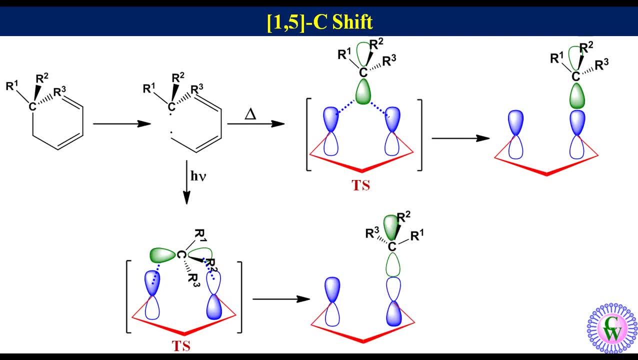 collapse into product that has the inversion in the configuration of the migrating group. 2. To summarize: under thermal condition, 1,5 carbon shift is supraphacial, feasible with the retention in the configuration of the migrating group, while under photochemical condition it is supraphacial and feasible, but with the inversion in the configuration.